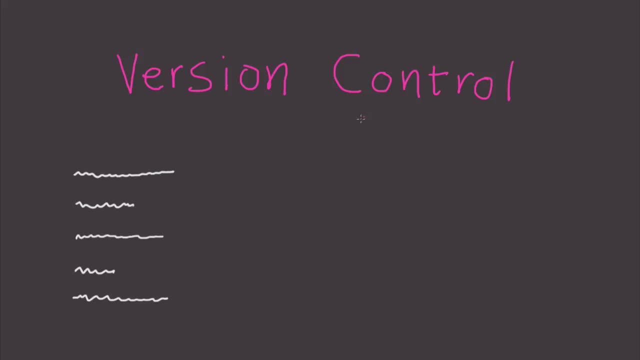 especially if you're a software engineer or if you want to get into software development, or if you simply work with files, whether you work with spreadsheet files, Photoshop images, Word documents, whatever it is, version control is a super useful thing. So let's get started and see what it is. 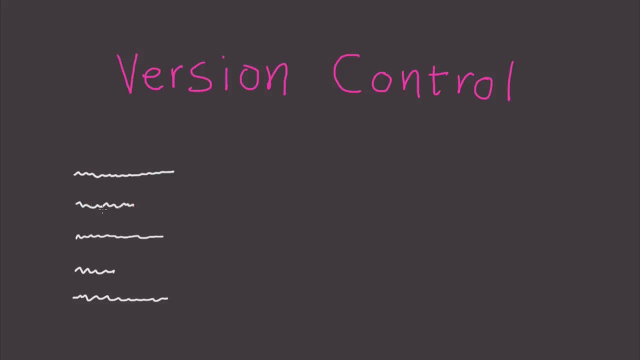 Let's say that I'm writing code or I'm just writing a Word document, So I've got a lot of lines and then I'm reviewing or I'm adding new lines, whatever. I decide that maybe take out this line And I save the file. I decide that maybe I want to rewrite this line. 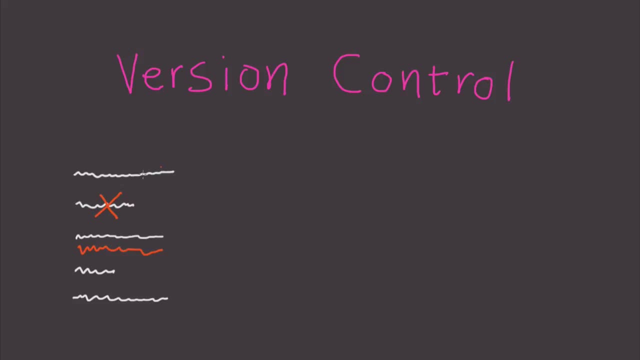 What happens is that every time that I make a change and I save the file, I lose the previous changes. So this is not a good thing. Maybe I'm working on a code and I had a working thing happening and now I try to add a feature and it's not actually working out to be a good idea. 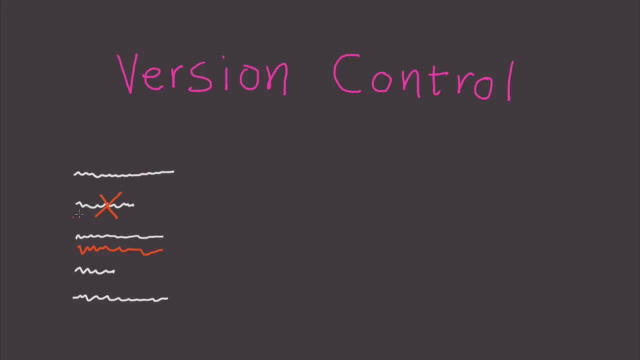 and now I lost my previous code. So if we're going to go like on traditional basis, then every time that you want to make a change you need to make a copy of your source code or of your Word documents before you make a further changes. 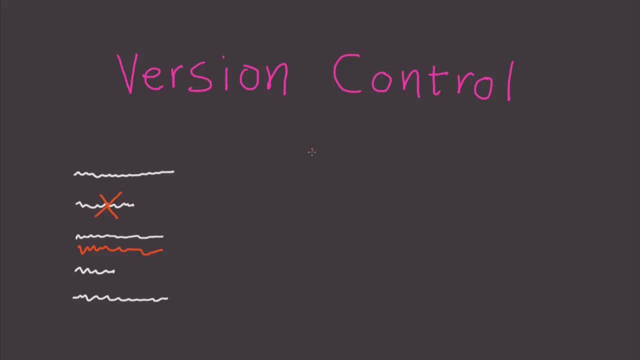 So that soon enough becomes a massive problem with a lot of files, and every time you save the file as a different name you need to stamp it with time and that becomes a massive mess. So what can we do to fix this problem? What if there is a special type of software that can monitor? 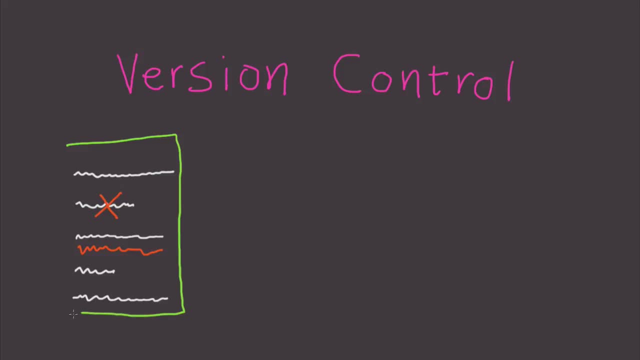 this file. So this file here could be monitored by a specific type of software, and this software can keep track of changes. So if you want to, for example, you start with the original, one original copy, and then maybe you want to go ahead and make some changes. 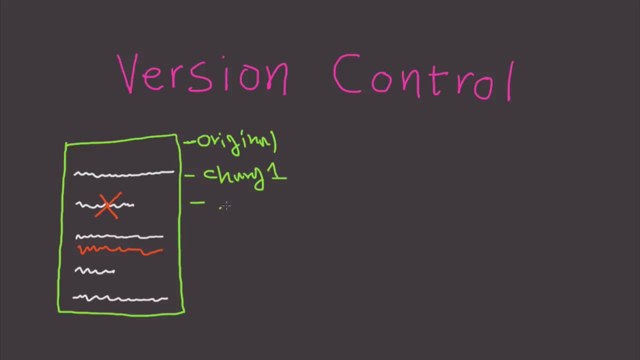 So this would be the change number one. You make some more changes, So on and so forth, And then you decide that, okay, there's all these changes. It was bad idea. So you want to go back to the original kind of file or any of these previous changes that you made. 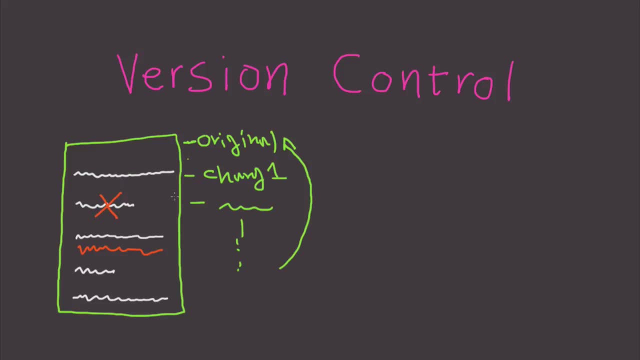 So that is version control. So basically it allows you to control different versions of your file. If you're working on a Photoshop file, it can monitor that file And every time you make a change you can basically commit. Commit is one of the words. 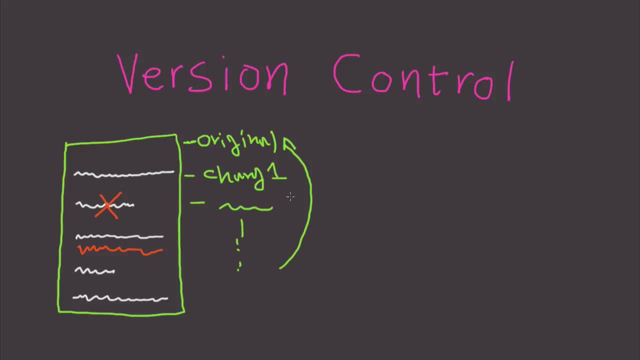 Which is used in the version control role, and you commit those changes to your branch. Branch is another term, So let's talk about what a branch is actually. So you have this file, you're working on it and we call this the current branch, right? 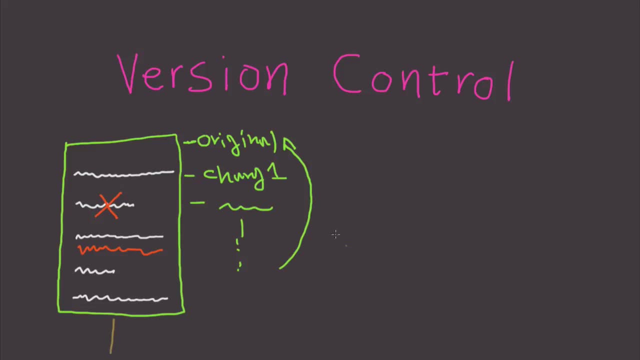 So this would be the current branch. Now let's say that you want to have another version of your file. Let's say that this current branch is a source code that you're working on to publish on Envato's marketplace. For example, my all-in-one iOS code that's on Envato for everyone to pick up. 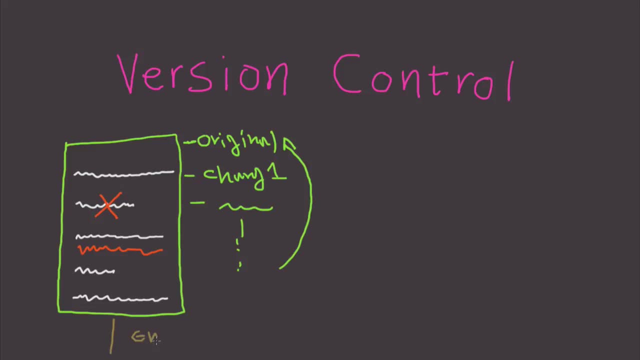 It's my maybe Envato's branch. I put it on Envato's branch Now maybe I want to do some modifications for myself, for my own use. So what I'm going to do is I'm going to make another branch and I would call this personal. 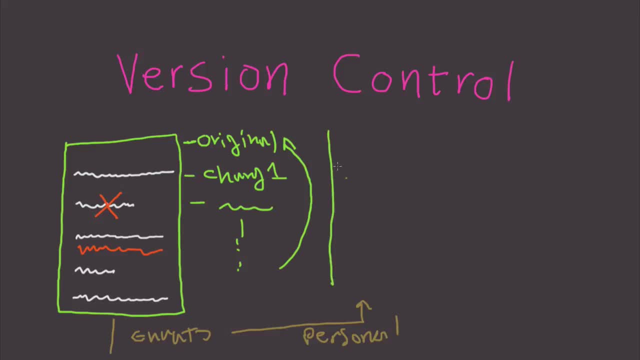 And I'm going to start modifying my own copy, My own kind of version of the file. So all the modifications that I make, it will happen on a separate branch and it's not going to affect my Envato's version. So every time that I make something different on the personal branch, it's going to stay. 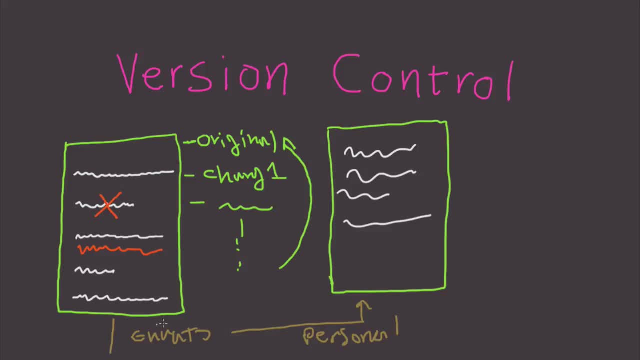 on the personal branch and I can just switch back to my Envato and do changes there. So I can have multiple branches of the same source code or a photo or a Word document on my system. Wow, And I only have one file on the system. 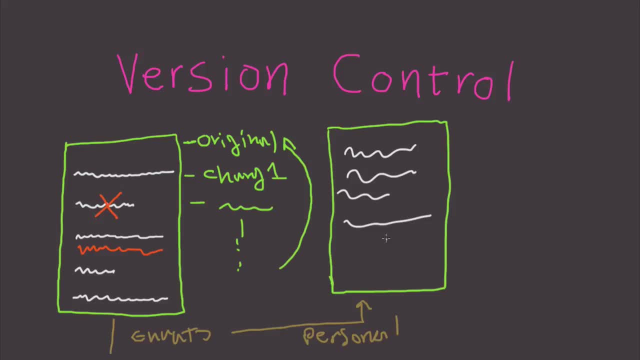 That's a very cool thing. There would not be a ton of different files that's going to clutter my desktop or my folders and I need to reopen all of them. All I need is just one local copy and the version control system keeping track of the. 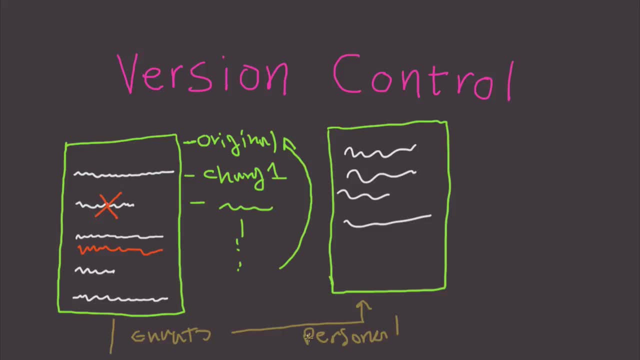 changes that I make, And every time I want to switch the branch, it automatically updates the file with the latest changes happening in that branch. So, as you can see, it's a very, very cool technology. Personally, I don't think modern coding or modern content producing would not be possible. 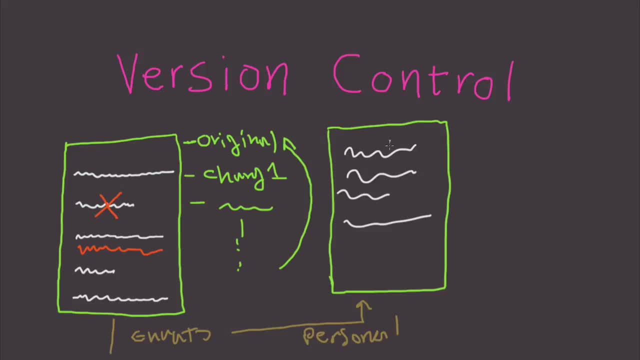 without it, with all these different changes that we make to our products. So how can you actually get this up and running? There are two technologies. First is Git. Git is the version control system that you install in your service, on your system. 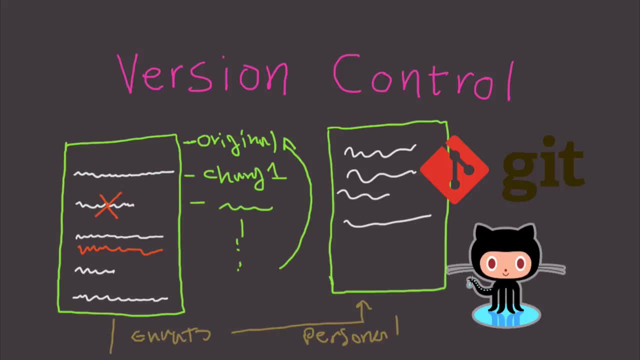 And GitHub is a social network. It's a social networking kind of service based on Git. So you use Git to kind of control your source code or photos or Word documents and then you can push it to GitHub as a public or a private repository or repo. 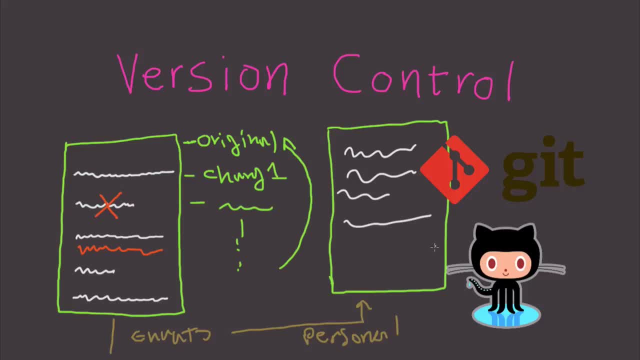 So you can make it public, so everyone else can use your code. Again, if you watched my open source video, this is a great way to share your open source code or open source content. If you want to share your code on GitHub, or if it's something that you want to keep. 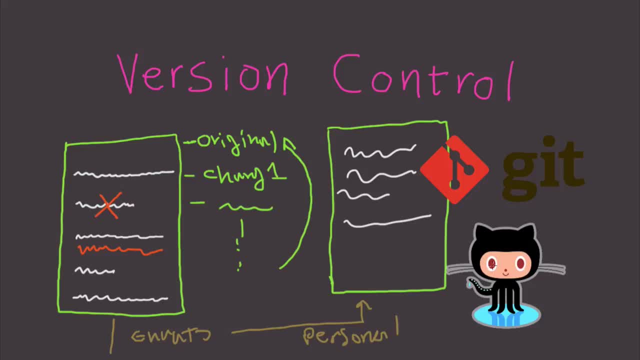 to your company or to yourself. you pay a monthly fee to GitHub and you share your code on GitHub on a private repo. So now you can see how powerful version control is and hope you're excited to use it. So if you enjoyed this video, check out this other video that I made, and it's full of. 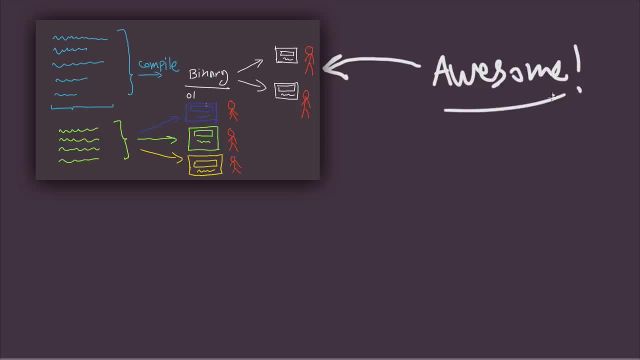 awesome content that you can learn in no time. Thanks for watching. I'll see you next time, As you did with this video. Also, if you think that you like my videos, then simply subscribe to my channel. I'm sure you're going to love the videos that I publish, if you like this one already. 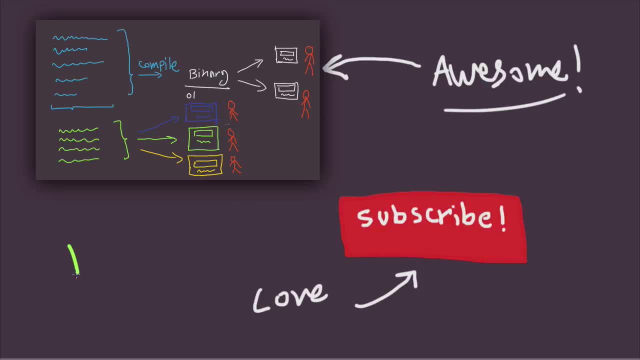 And I'll be seeing you in the next video. Thanks for watching Hooman's here and have a good day.